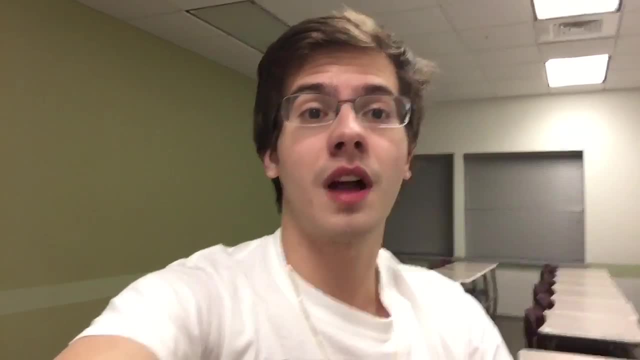 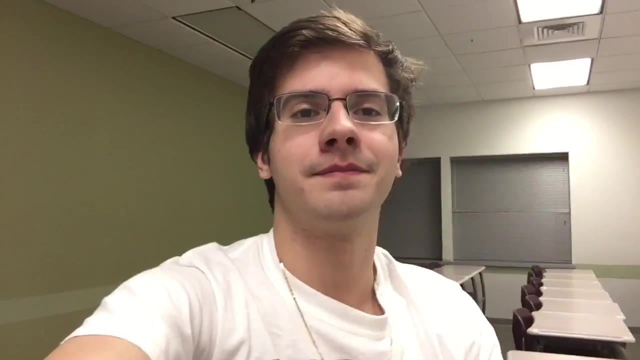 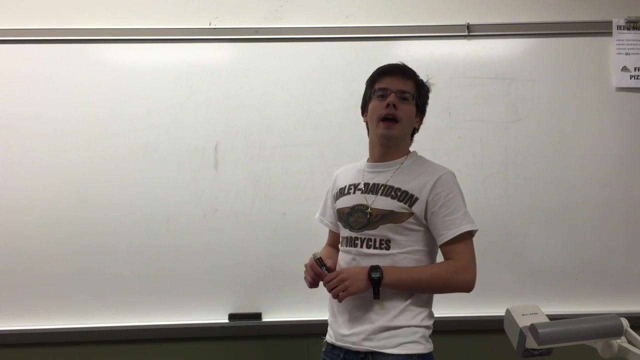 Hi everyone. so in this video I'm going to talk about four kinds of differential equations that you need to be able to identify them and solve them. I hope you enjoy. In this video I'm going to give you an overview of what these four types are and the methods that we could use to identify them and solve them. 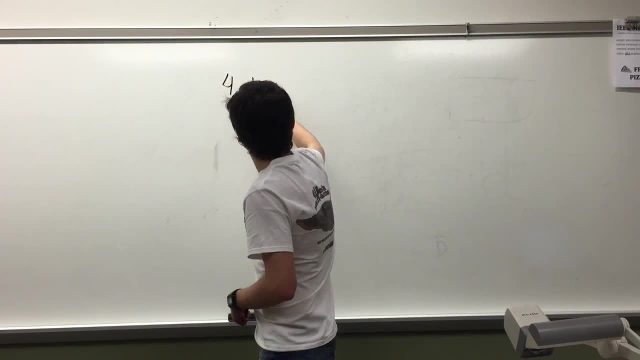 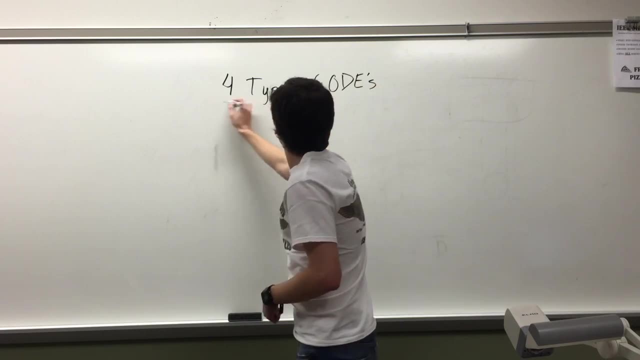 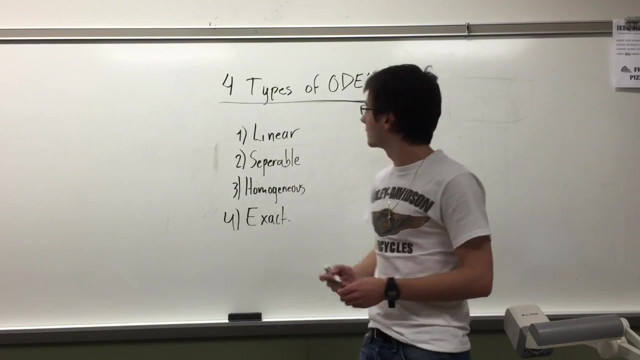 So the four types of ODEs that we have is linear, separable, homogeneous and exact. So let's talk about the first one. A linear ODE is given in the form y prime plus p of t times y is equal to g of t. 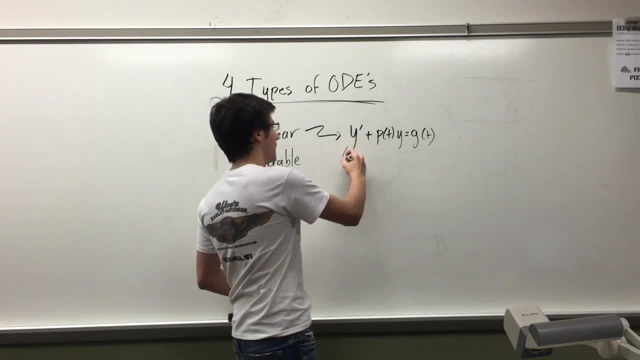 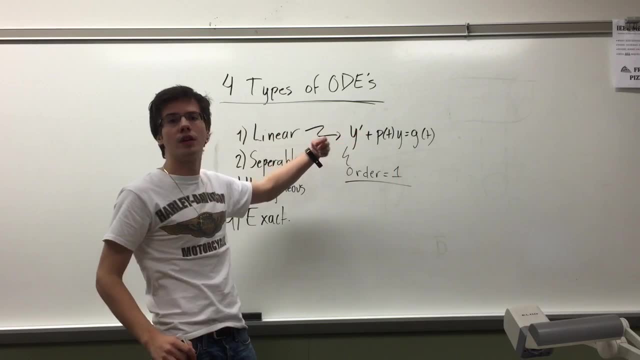 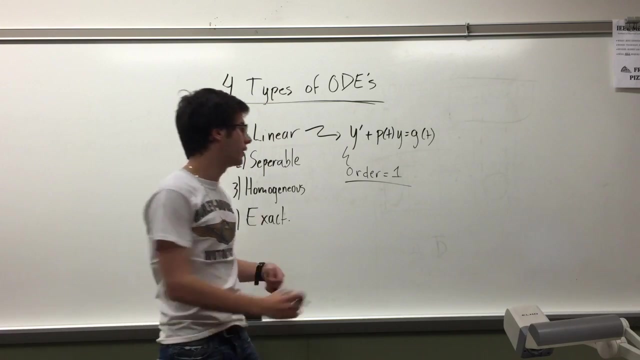 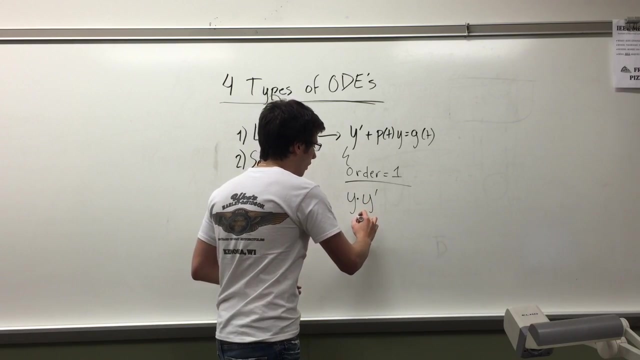 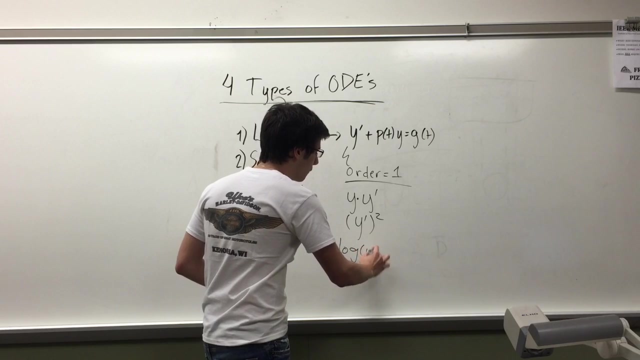 This is the form of a linear ODE because it has the order of one, because it's only the first derivative, So it has an order one and it doesn't have any of the special cases that we talked about in the previous video, where we can't have the function times its own derivative or the derivative squared or anything like a function of the derivative, like log of y or y prime. 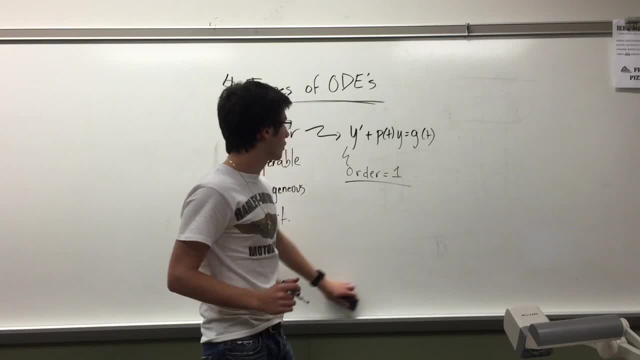 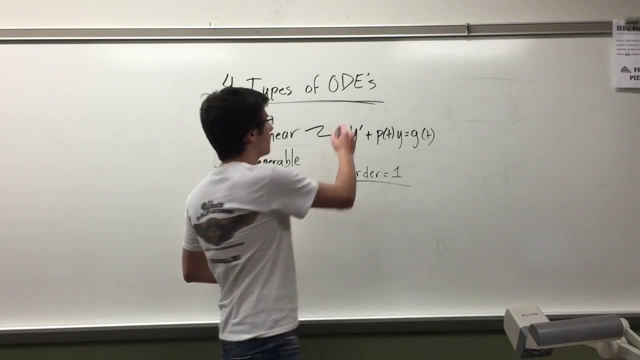 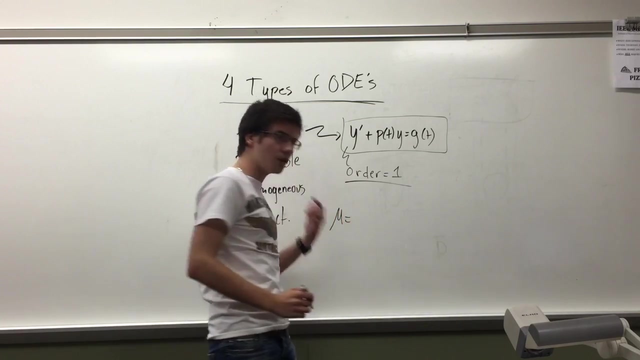 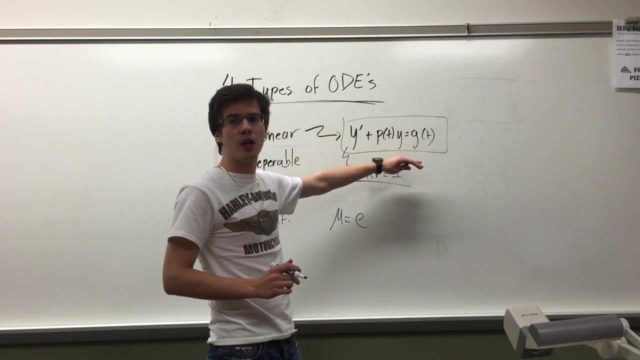 These can't happen in a linear ODE. So we usually see, we can identify a linear ODE E Easily by sight if it has the following form: and how do we solve them? We solve them by using the integrating factor. So this genius, genius mathematician, he was able to figure out an expression that if you multiply this expression by differential equations and you use some some calculus tricks by using the product rule, 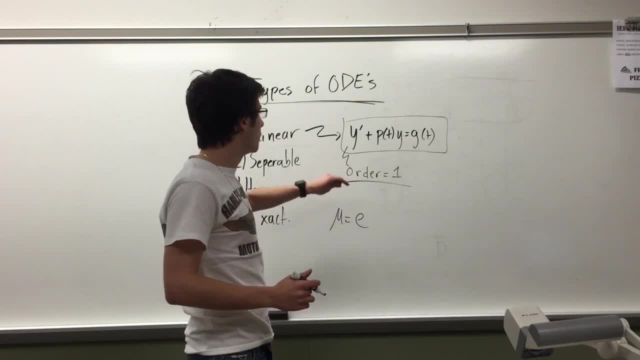 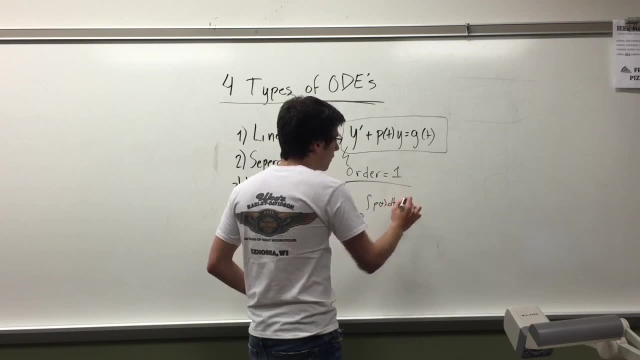 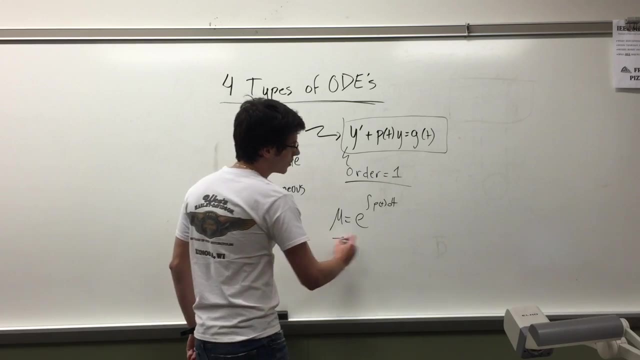 You get, You're able to find a solution to your ODE. So very smart trick, And we're going to go more in depth in another video going through the whole derivation and solving more examples to this, But simply this is what's called the integrating factor. 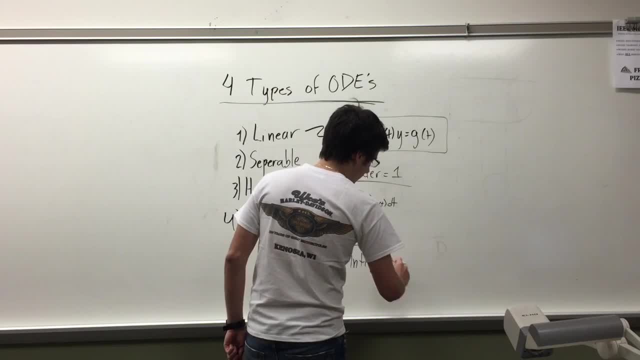 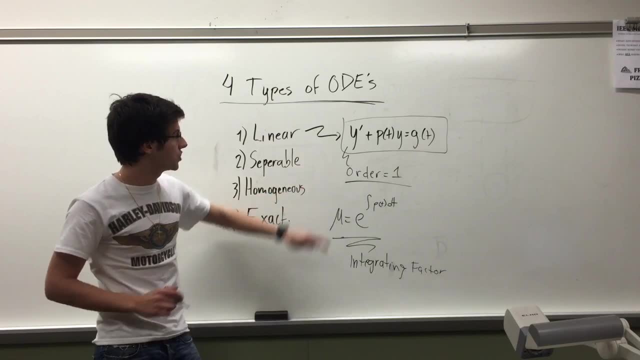 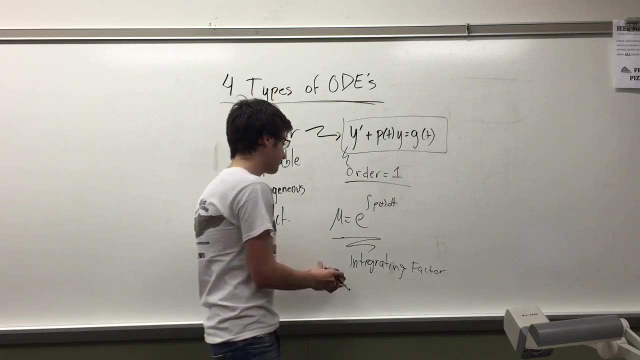 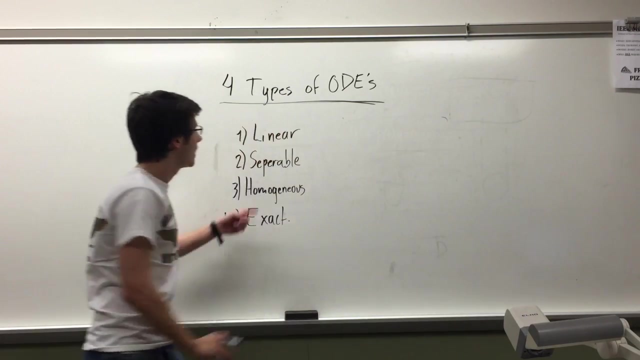 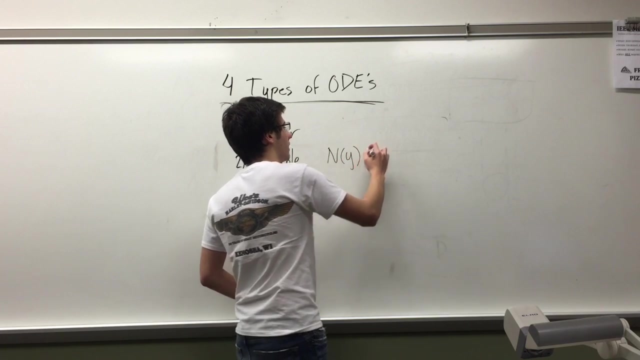 Integrating factor to great Integrating factor, And this is what we use when we have A linear ODE. we just multiply it by the ODE, use the concept of product rule and we're able to solve it All right. now let's talk about the second type of differential equation. the second type is a separable ODE. a separable, separable ODE has the form n of y times d, y, d, x is equal to n of x. 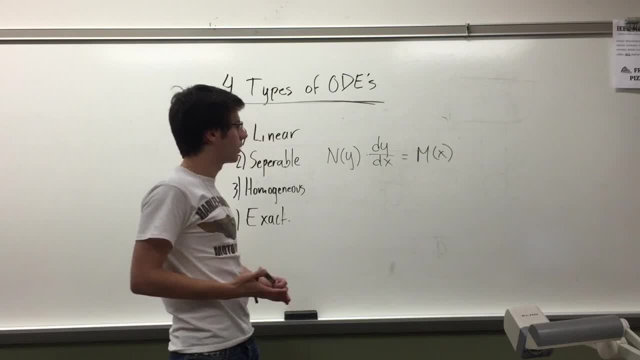 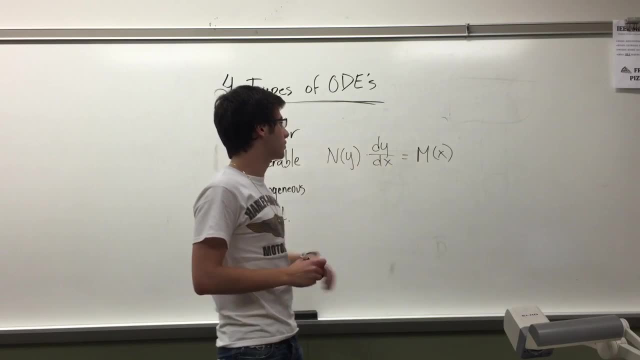 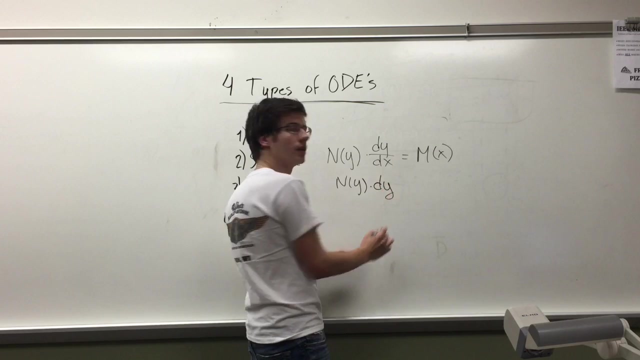 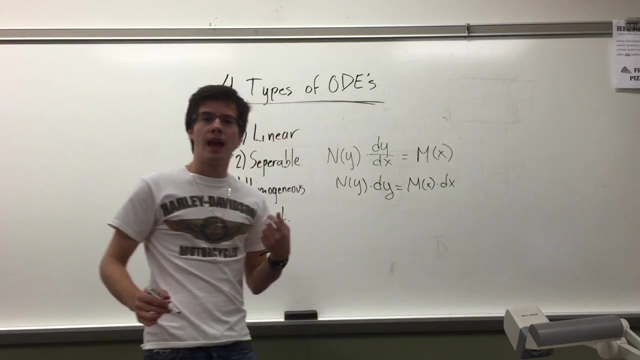 So Basically It's hard to understand this form right off the bat, but basically it says that a function of y times its derivatives is equal to a function of x, or in other words, we could write that a function of y times its differential d y is equal to a function of x times its differential d x. 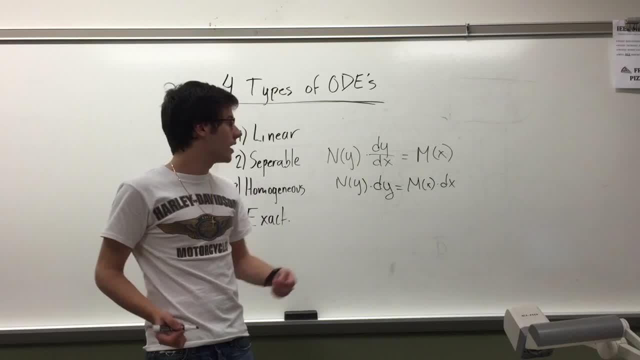 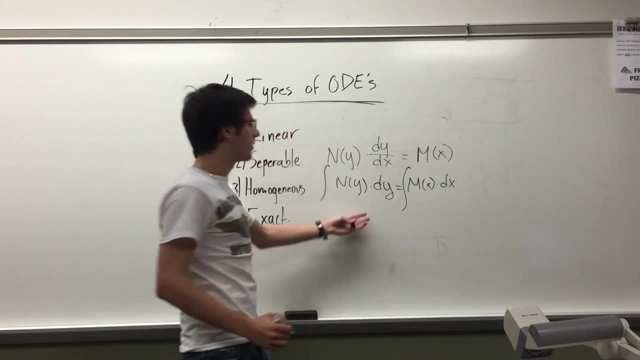 And the reason why it's so nice to have these kind of ODE is because this is in function of y, This is in function of x, so we can simply integrate both sides and then we can find our solution. So, basically, separable differential equations. 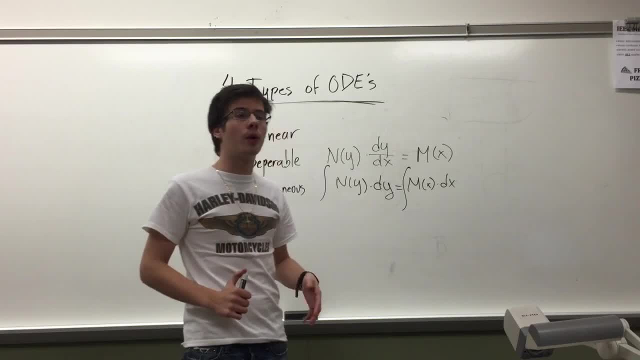 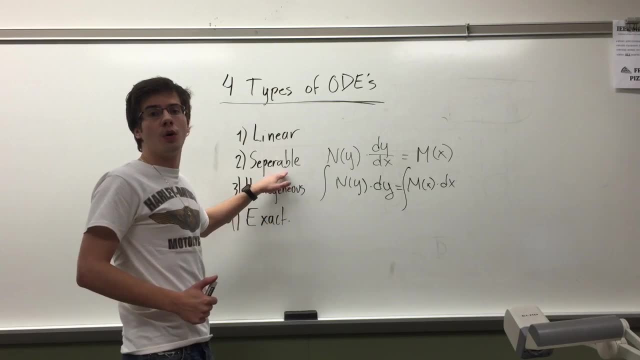 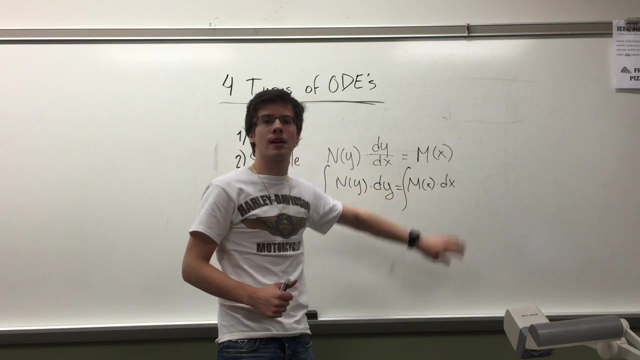 We can identify them by trying algebra, we try to factor it out and have and separate the variables. that's why it's called a separable ODE, because we're able to separate the variables into function of y and this side, function of x and this side. 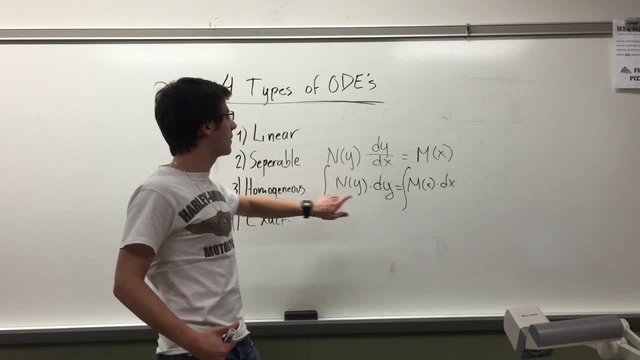 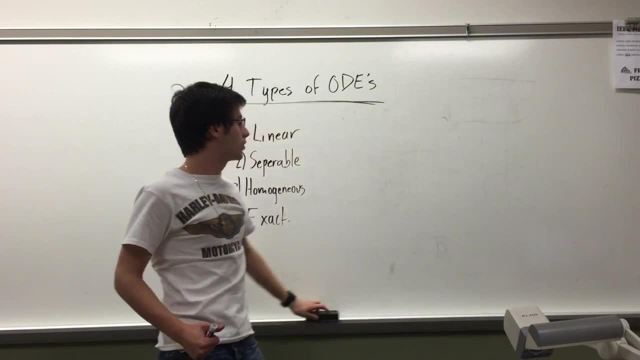 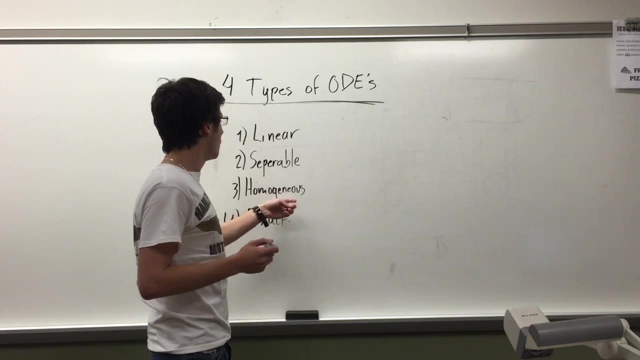 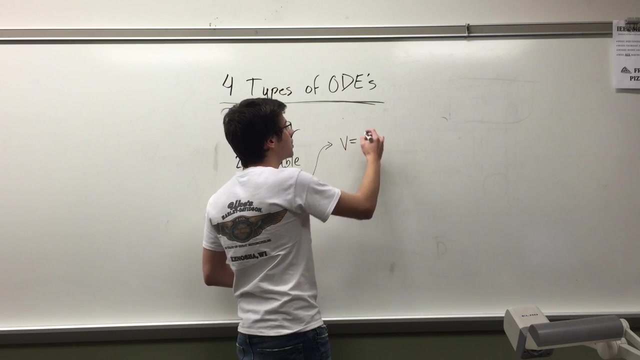 And then Our strategy to solve them is to simply integrate both sides and then we can easily find a solution. The last two are kind of hard to talk about in in this brief overview that I'm giving, but homogeneous is basically. our strategy of solving homogeneous equations is that we're going to do a substitution of v equals y over x, and when we do the substitution,